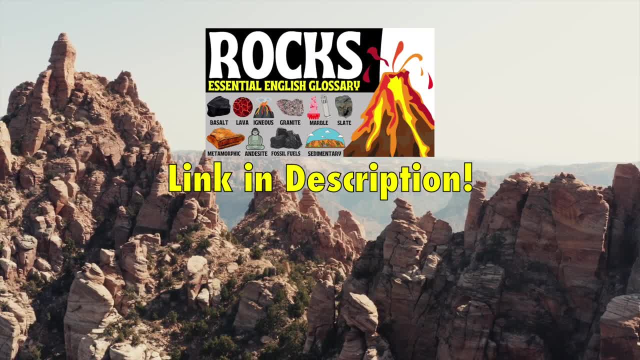 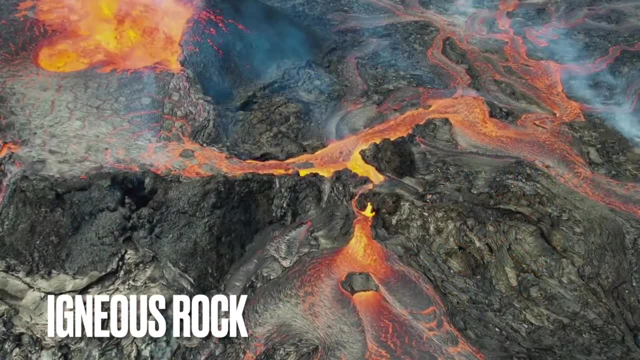 you should check out my video on rocks, where you'll discover lots of additional useful vocabulary. Let's move on to igneous rocks. These are another fundamental type of rock that form from the cooling and solidification of molten magma or lava. They can be considered to be: 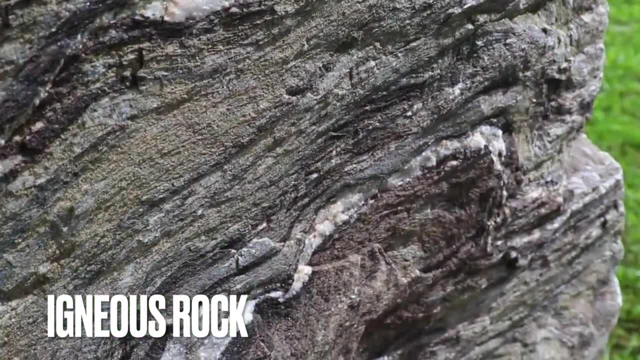 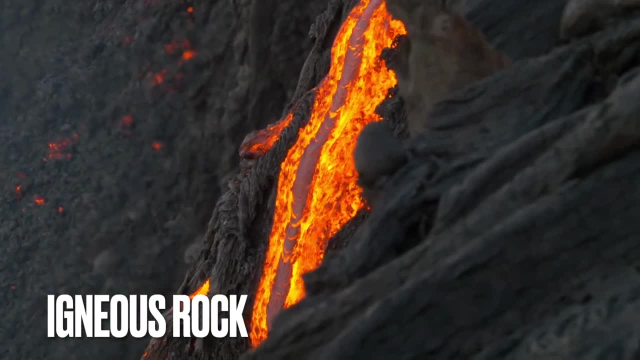 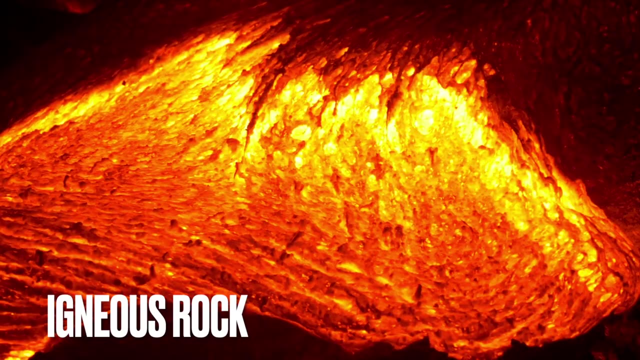 a solid rock. They can be categorized into two main types: intrusive or plutonic, which forms below the earth's surface and has coarse grained textures. The other type of igneous rock is extrusive or volcanic. These rocks form on the surface and have fine grained textures due to 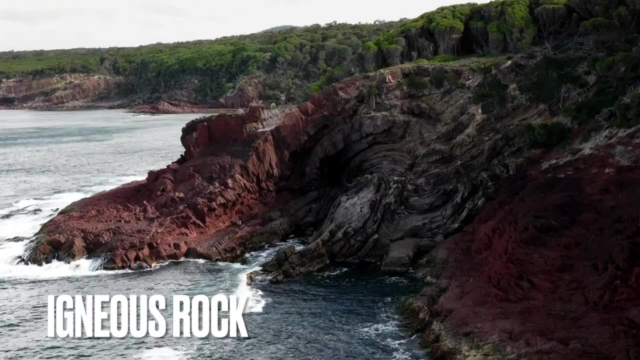 rapid cooling. Igneous rocks vary in composition from felsic to mafic, influencing their color and mineral content. Our next category of rock is a rock that forms on the earth's surface and has coarse grained textures. These rocks can be categorized into two main types: intrusive or plutonic, which forms 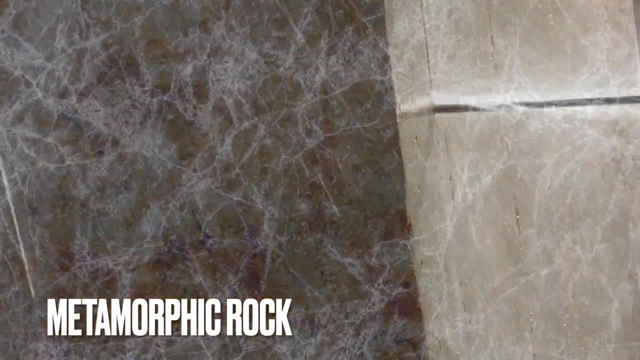 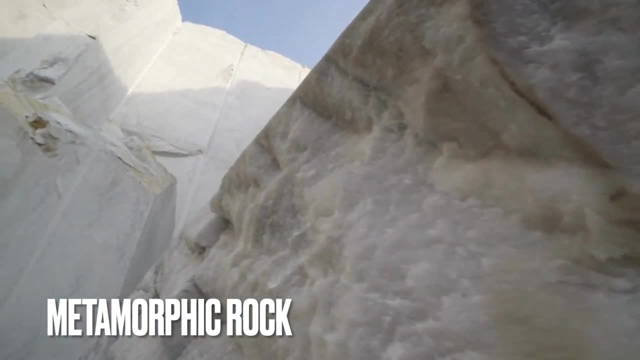 below the earth's surface and has fine grained texture. The other category of rock is metamorphic. Metamorphic rocks are a significant category of rocks that form from preexisting rocks, either igneous, sedimentary or other metamorphic rocks, and this happens through intense heat. 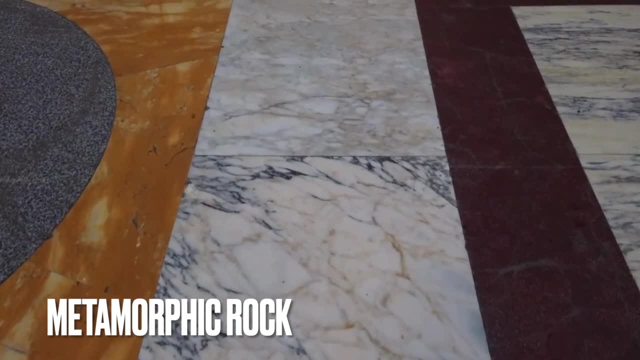 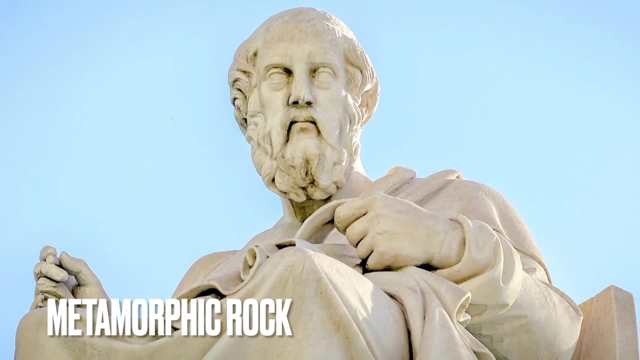 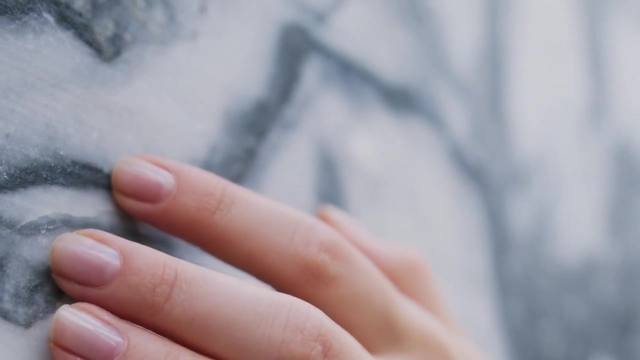 pressure and chemical changes within the earth's crust. These transformative processes cause the original rock to recristallize, resulting in new textures and mineral compositions. Metamorphic rocks often exhibit foliation, which is the alignment of minerals in parallel layers, giving them a banded appearance. 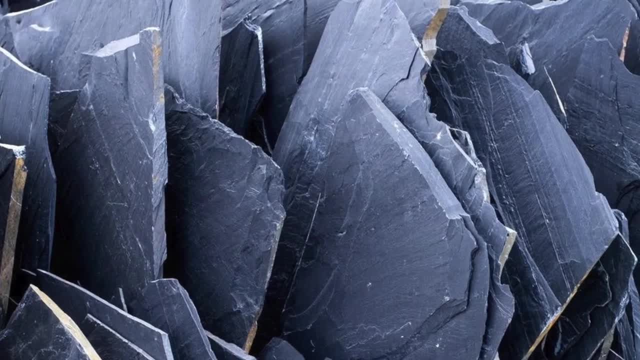 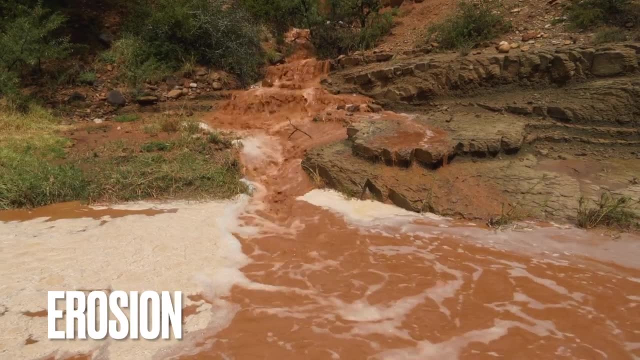 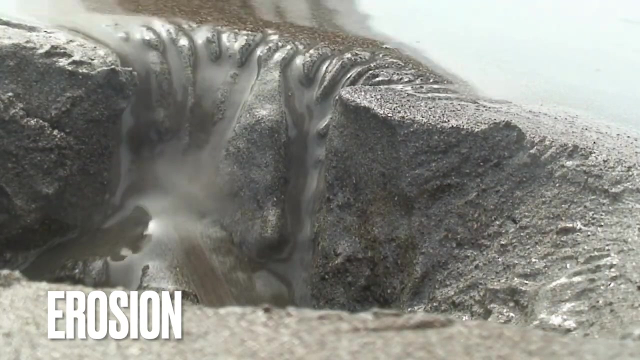 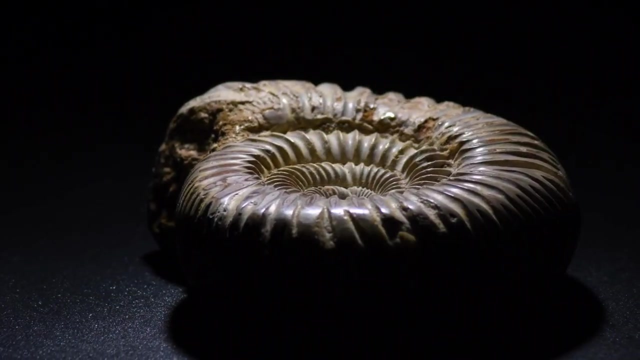 Examples of metamorphic rock include marble and slate. Let's move on to a really important term in geology: erosion. Erosion is the process of wearing away and transporting rocks and soil by natural forces like wind, water or ice. Another really important term, and something you may have heard me already mention in the video, is a fossil. 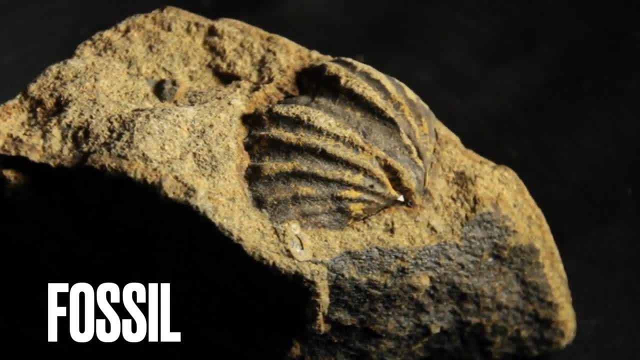 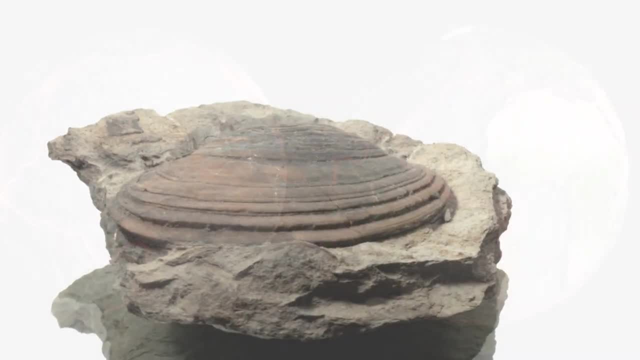 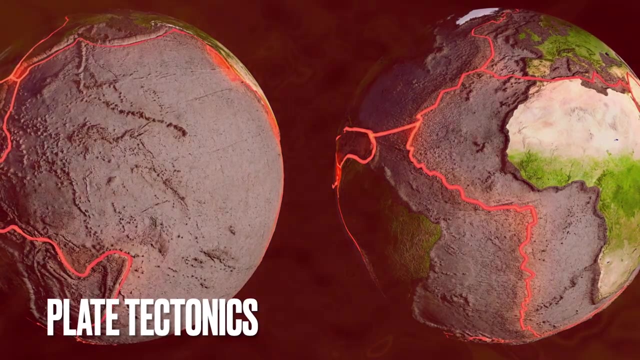 A fossil is the preserved remains or traces of ancient organisms. Fossils can tell us a lot and can provide valuable insights into Earth's history. Another term I referenced earlier was plate tectonics. Plate tectonics is a foundational theory in the field of geology. 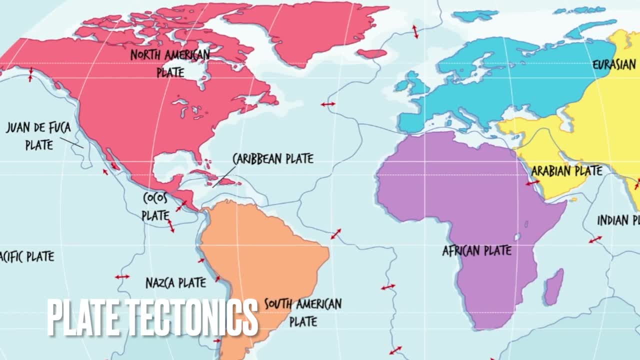 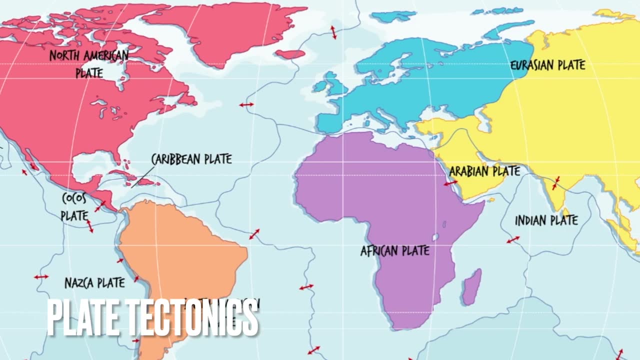 that explains the importance of the use of plates in geology. Plate tectonics is the dynamic movement of the Earth's lithosphere, which consists of large, rigid plates that float on the semi-fluid athenosphere beneath them. These plates are in constant motion, driven by the heat generated from the Earth's interior. 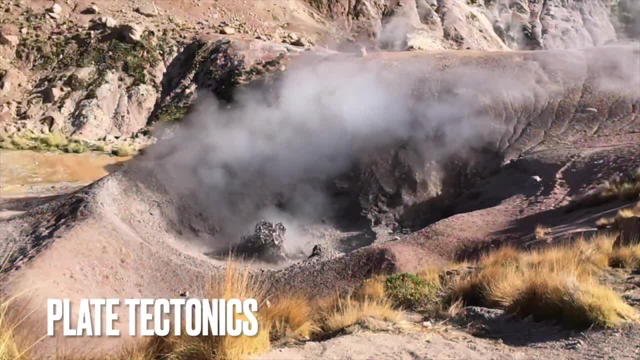 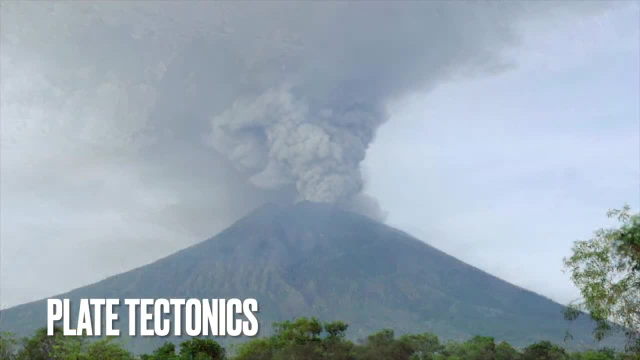 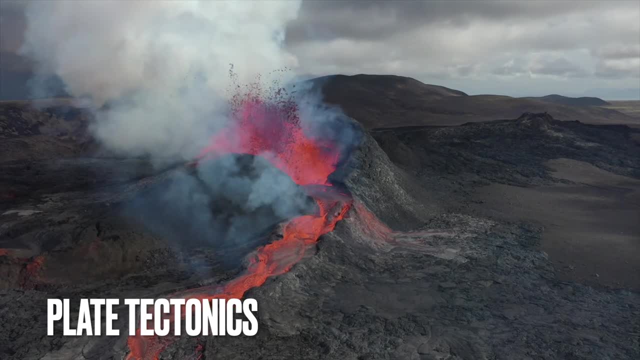 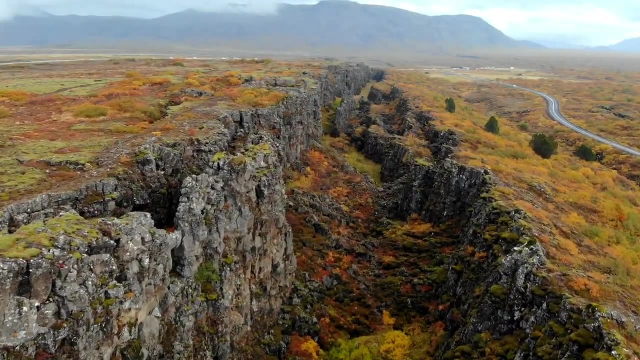 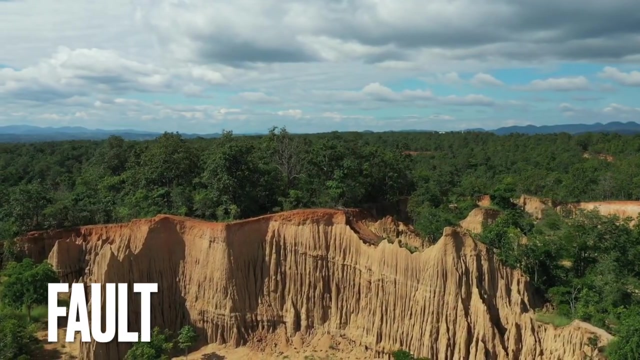 and provides insights into the formation and breakups of continents, the distribution of earthquakes and volcanoes, and the processes that shape our planet's landscape over geological time. A feature of plate tectonics is a fault. This is a fracture in the Earth's crust along which movement can happen. 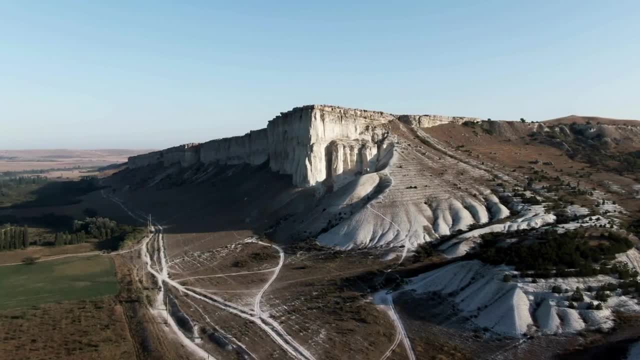 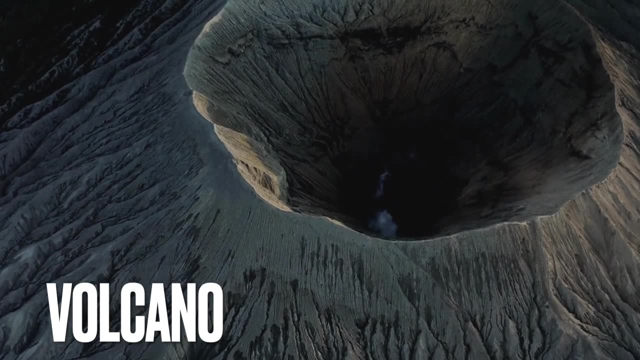 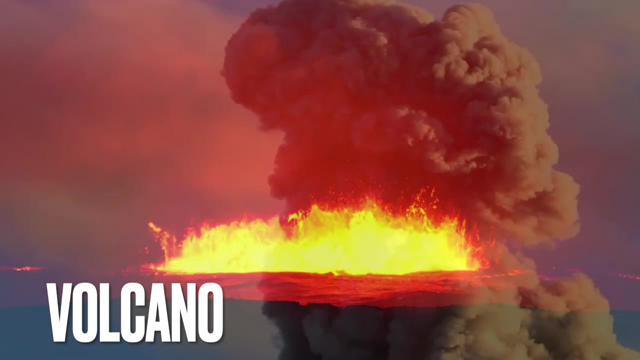 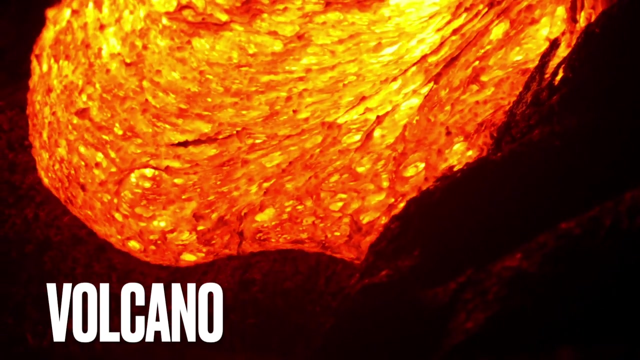 These often cause earthquakes. Volcanoes are geological features that result from the eruption of molten rock, ash and gases from the Earth's interior onto its surface. They happen at specific locations known as volcanic vents or openings in the Earth's crust. Volcanoes can take various forms: from towering mountains like Mount Fuji, 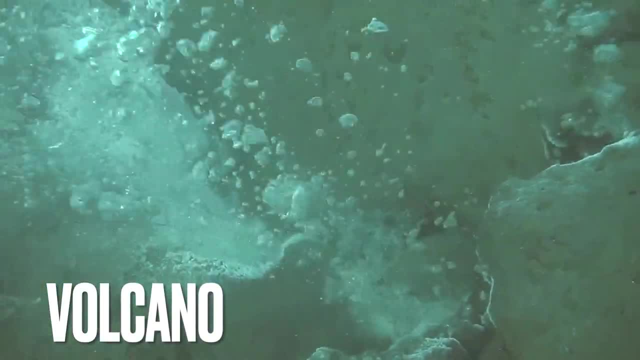 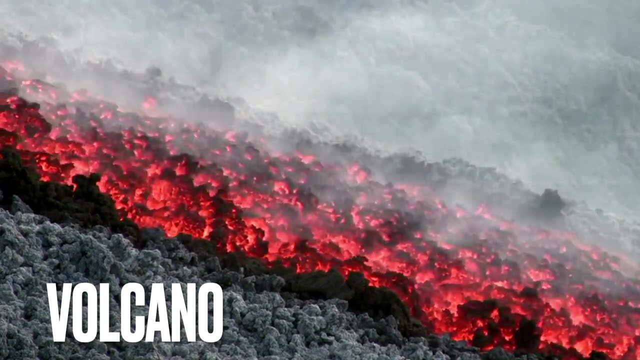 to underwater vents on the ocean floor, The eruptions can be explosive. Volcanoes can be explosive or effusive depending on the type of magma involved and the presence of gases. Volcanic eruptions played a crucial role in shaping the Earth's landscape. 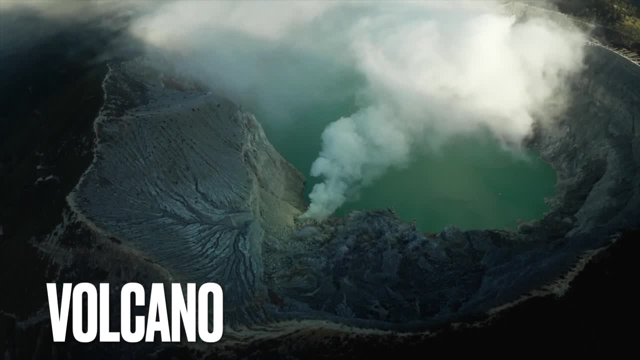 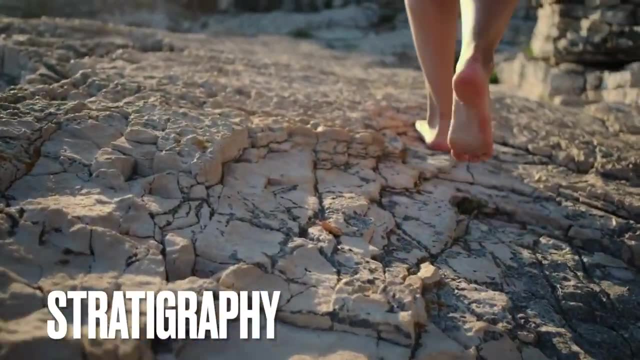 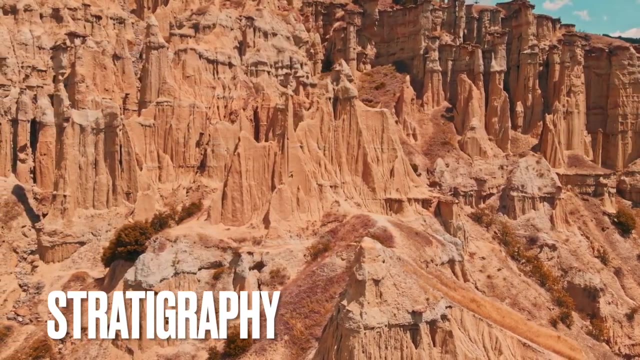 and can have significant impacts on the environment and human communities. Stratigraphy is a branch of geology that focuses on the study of rock layers or strata and their arrangement in chronological order. It plays a crucial role in the development of geological structures. It plays a crucial role in deciphering Earth's history. 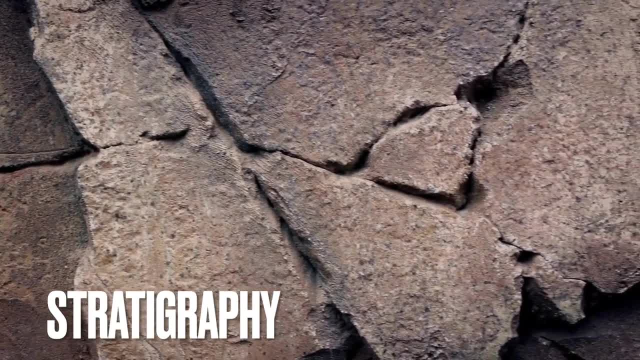 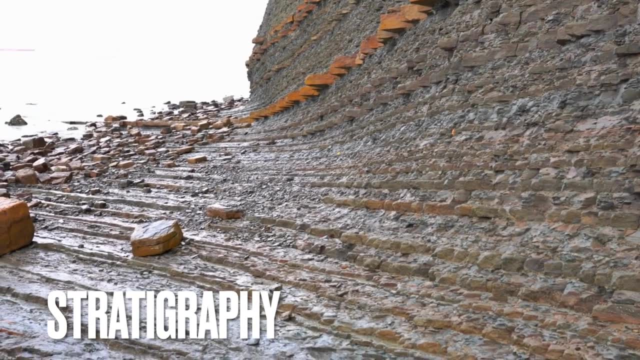 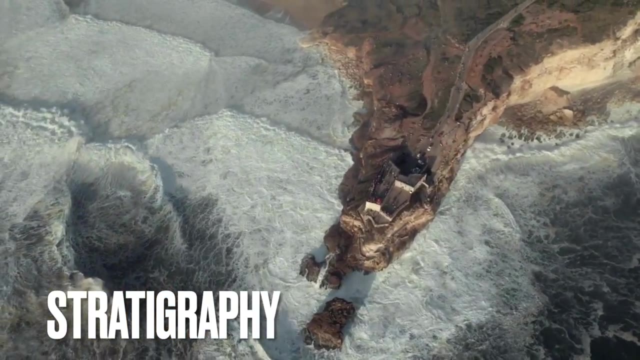 and understanding the sequence of geological events that have shaped our planet. Stratigraphers examine the characteristics of these layers, including their composition, fossil content and relative positions, to determine the relative ages of rocks and the events that have happened over millions of years. 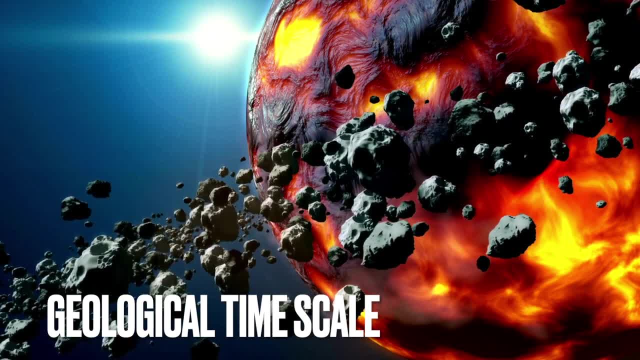 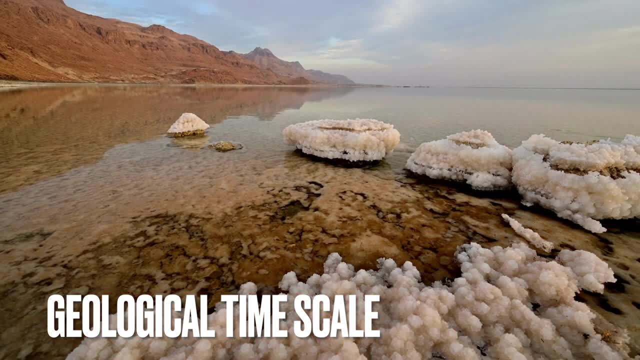 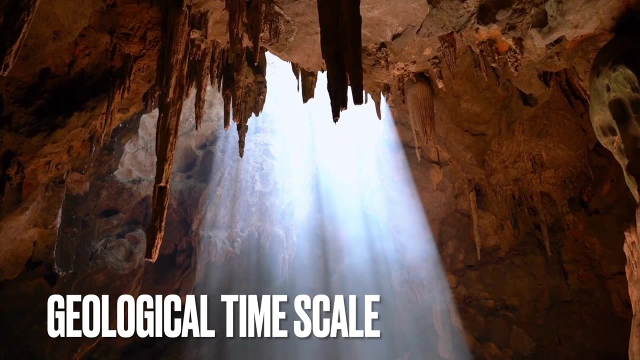 When we're talking about millions of years, we're talking about a geological timescale. This is the framework used by geologists and paleontologists to divide Earth's vast history into distinct periods, epochs and eras, helping us understand and organize the sequence of geological events. 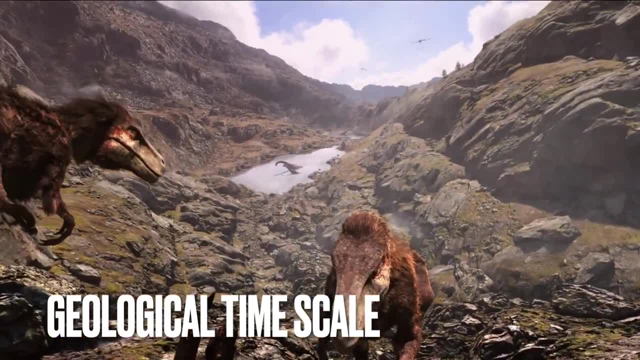 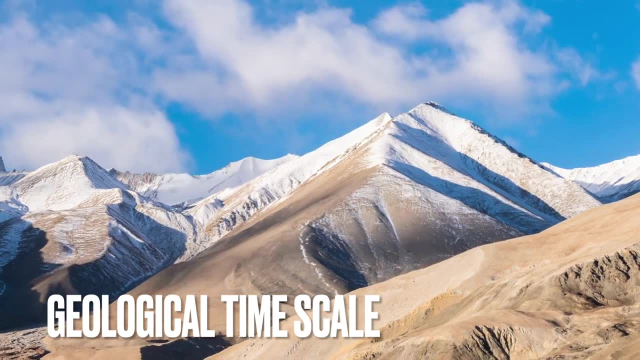 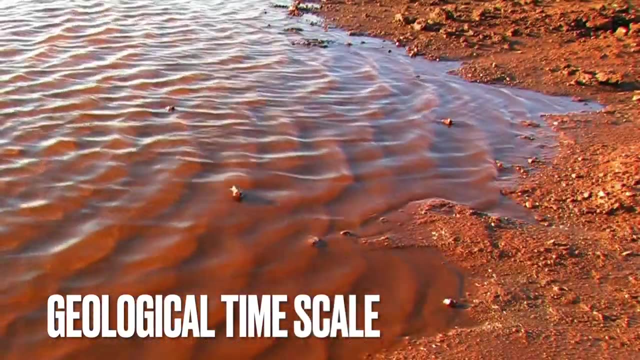 and the evolution of life on our planet. It is divided into eons, eras, periods, epochs and ages, each representing specific intervals of time. The largest divisions, eons, encompass billions of years, while the smallest ages represent shorter intervals. 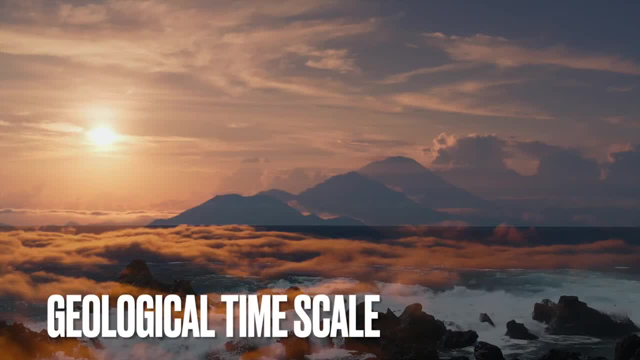 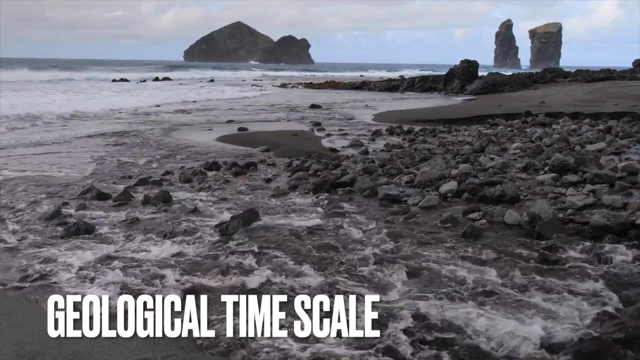 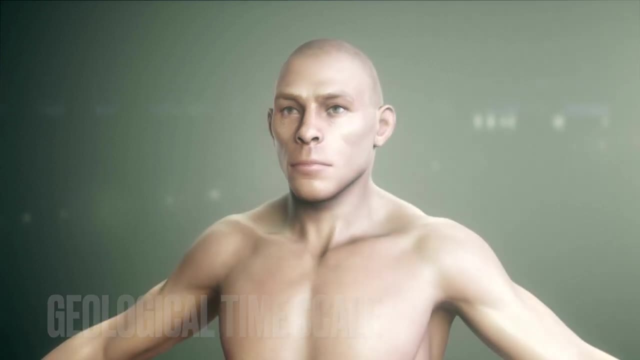 Notable divisions include the Phanerozoic Eon, which covers the last 540 million years and includes the Paleozoic, Mesozoic and Cenozoic eras, during which major life forms have evolved and geological events have happened. 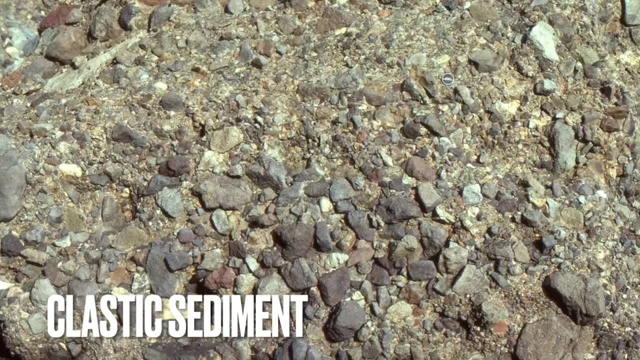 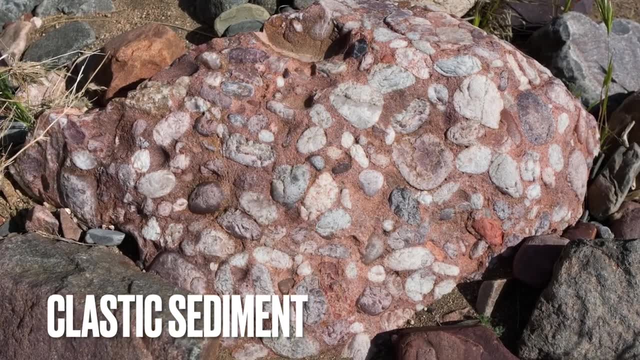 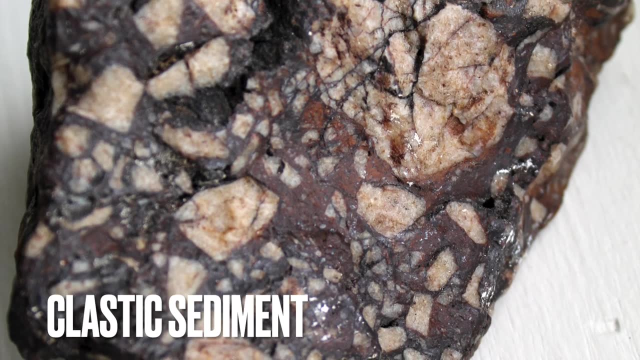 Our final term for our geology lesson is Clastic Sediment or Plastic Sediment. This refers to a type of sedimentary material composed of fragmented pieces of pre-existing rocks and minerals which are transported by natural agents like water, wind or ice and then deposited. 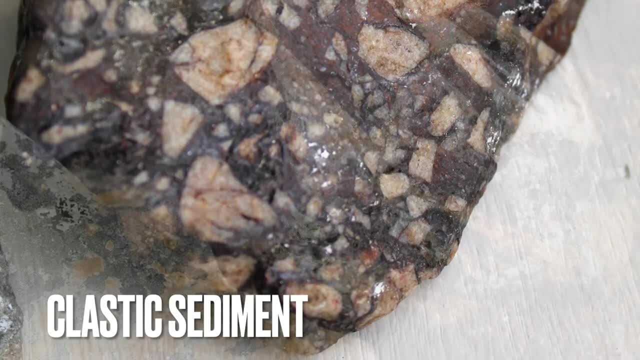 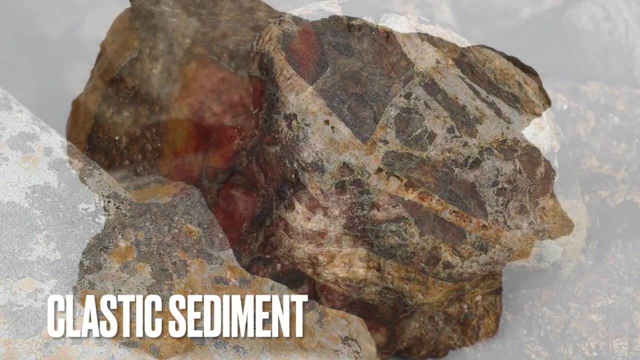 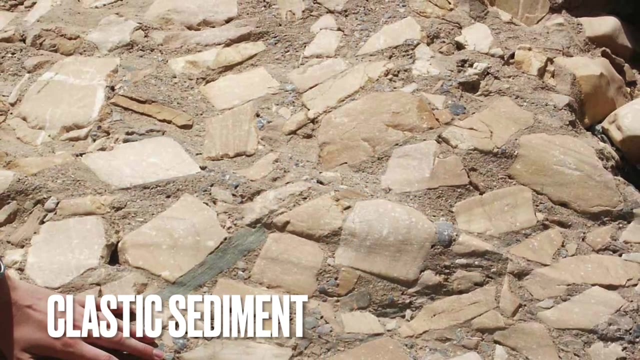 Clastic sediments can vary in size, from tiny clay particles to larger sand, silt or gravel-sized fragments. The classification of clastic sediment is often based on the size of these particles, with categories including clay, silt, sand and gravel. 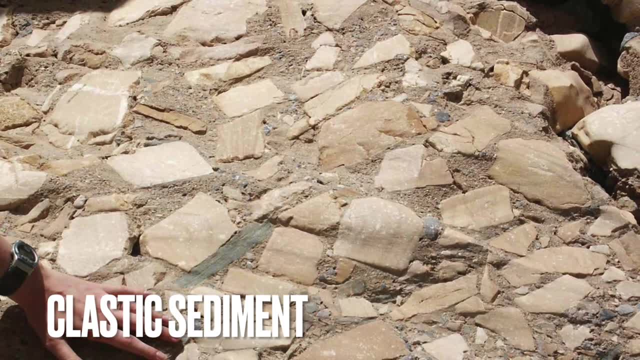 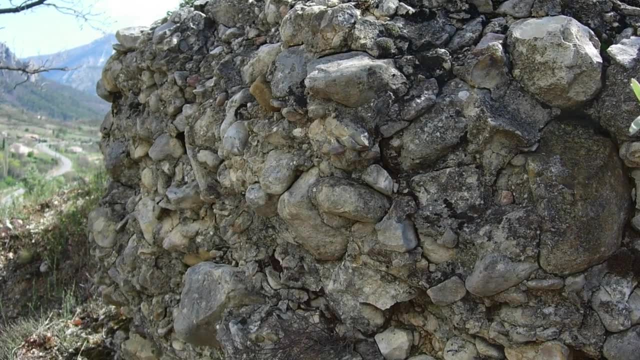 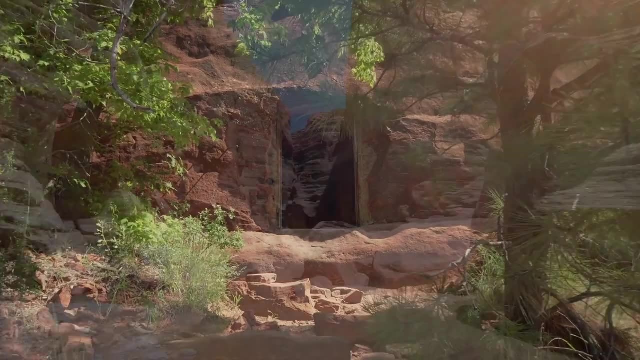 Over time, these sediments can accumulate and become compacted and cemented together, eventually forming clastic sedimentary rocks such as sandstone shale or conglomerate. And there you have it: we've covered lots of essential geology terms that are sure to kickstart your journey into the captivating world of geoscience. 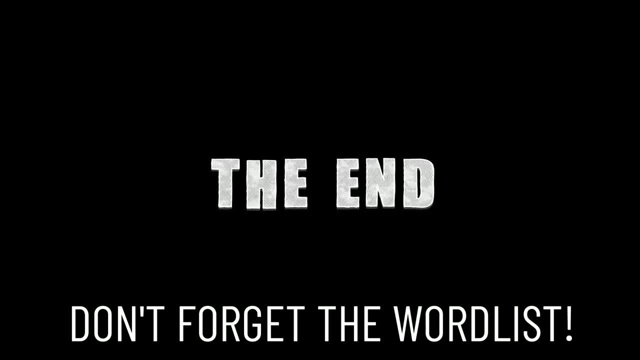 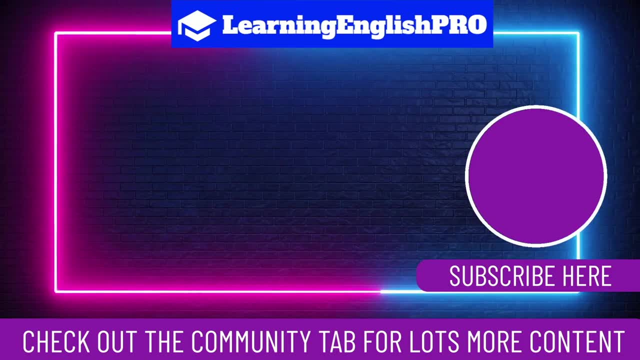 If you found this video helpful, don't forget to like, share and subscribe to Learning English Pro for more educational content, And on screen are some links to some similar videos which might give you an additional boost in your geology studies. As usual, have a great day and remember. keep learning English like a pro.